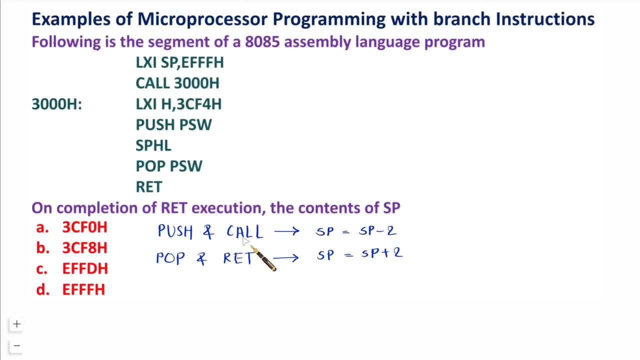 explained. when you perform call execution at a time microprocessor that will push content of main program, which is there with program counter on stack. For that it will have to push stack pointer Right. That's why stack pointer will get decremented by 2.. And when you perform return, 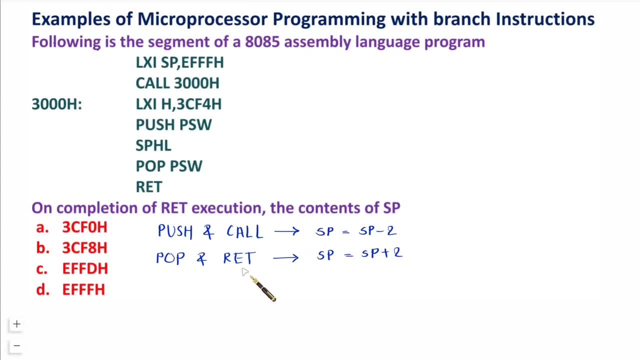 instruction. at that time, microprocessor will retrieve original program's location, which was there on stack, by performing pop instruction execution inside Right. So that is how push and call that will be executing stack pointer. Now, my dear students, I'll explain you how to do this. 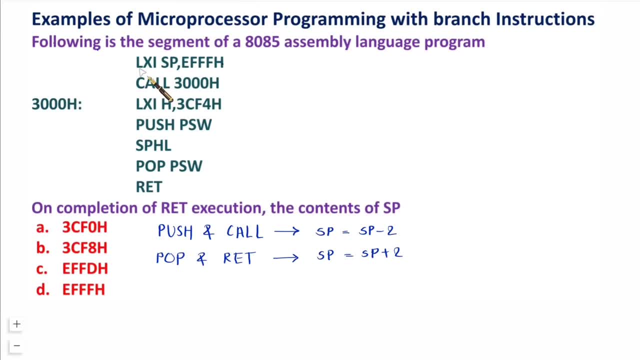 This program step by step. So first of all let us execute LXISP, EFFF, hex. So what will happen? stack pointer. now that will be equals to E, F, F, F, hex. After that we perform: call 3000, hex. So here we have 3000 hex. So here we will be providing subroutine. But what? 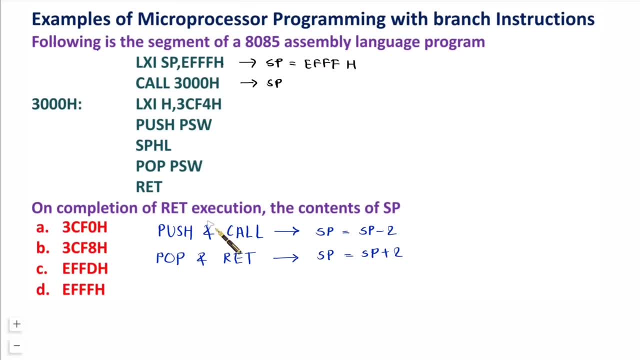 will happen with stack pointer. my dear students, Stack pointer in call, it will get decremented by 2.. So initially it is this, Now it will decrement by 2.. So now it will be E, F, F and F minus 2, that will be D. Now let us execute this instruction. Now we have provided subroutine. 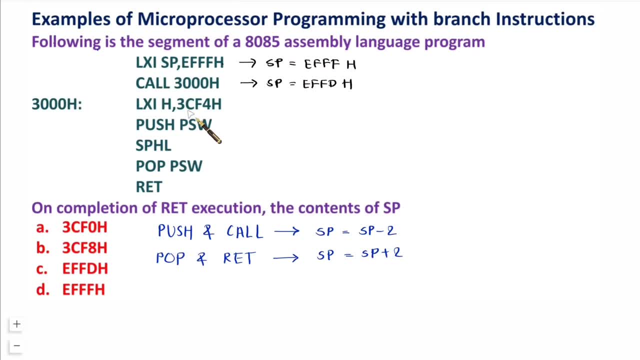 here. So here LXISP 3C F4 is there. So now HL pair. now that we are changing to 3C F4, hex Means we are loading HL pair with this data. Now we perform push PSW. My dear students, I 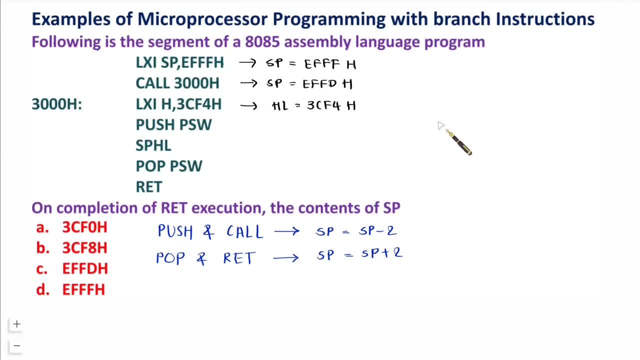 don't know what is accumulator and flag resistor. You should know PSW, that is a combination of accumulator plus flag resistor. Right, So here we don't know this. Right So here question is based on stack pointer, only, Right. So when you perform push, you should know stack. 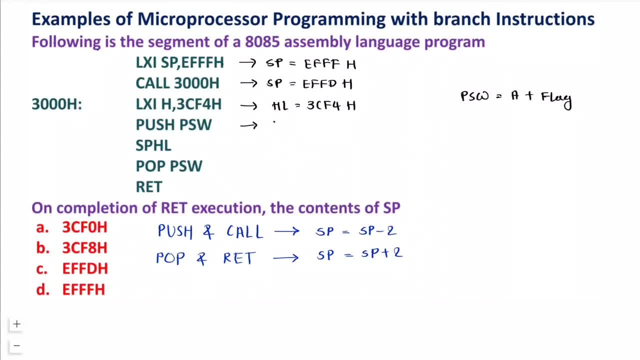 pointer that should get decrement by 2.. So here we perform push PSW. Now we perform push the stack pointer. So here, stack pointer that was E, F, F, D, Now it will get decrement by 2.. So now it will get to E, F, F, D minus 2, that will be B hex. Now we perform SPHL. 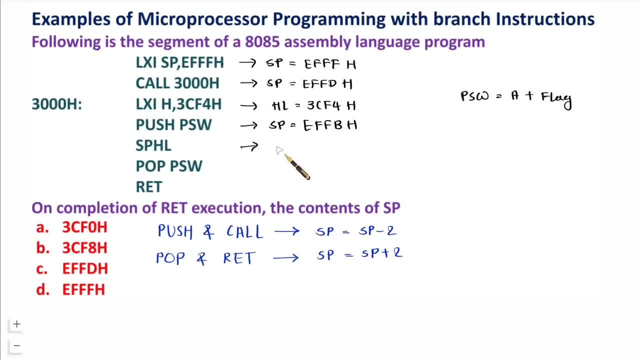 My dear students, this instruction is very interesting. You see, HL pair and stack pointer that will exchange their data with each other. Right HL data is 3CF4.. Now that will go in stack pointer and stack pointer data. that will go in HL. 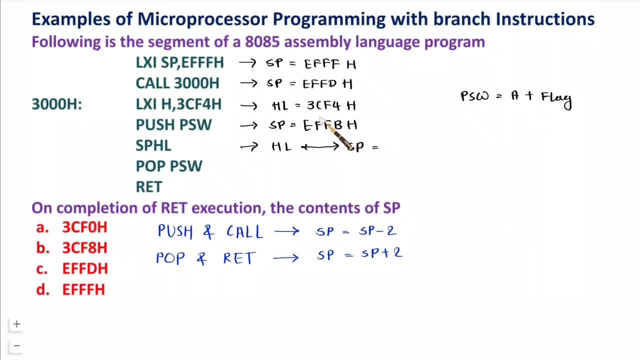 So now stack pointer will get modified to this data which is there with HL, So that is 3CF4, hex. Now, my dear students, we perform POP, PSW. So you see, now, when you perform POP, at that time stack pointer will get increment by 2.. 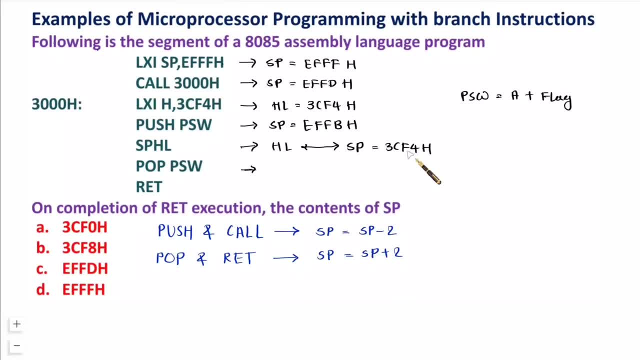 So before this instruction stack pointer was 3CF4.. So now stack pointer, it will get increment by 2.. So now it will be 3CF4 plus 2, that is 6 hex. After that we perform return instruction. 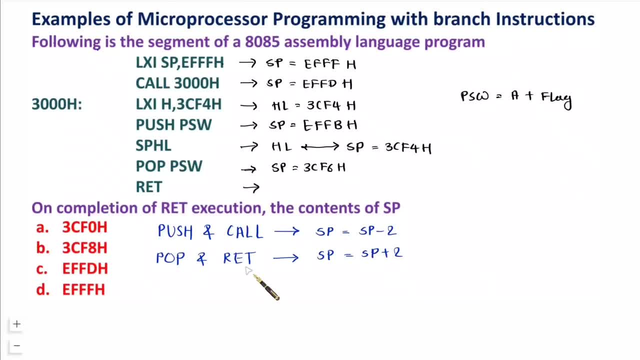 So stack pointer again, it will get increment by 2,, right, So stack pointer now it will get modified to 3CF8 hex after return execution. So in option you see this is our correct option, right So? So that is how we can be able to solve question based on push, POP and call return instruction. 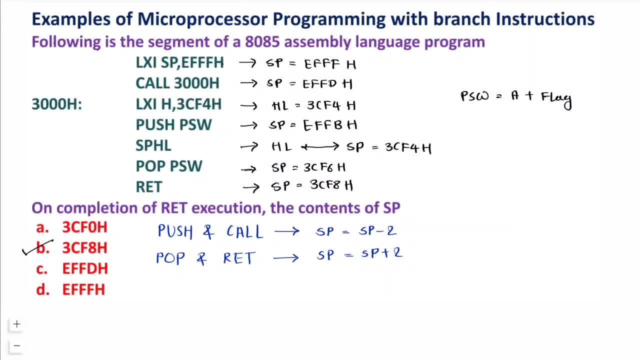 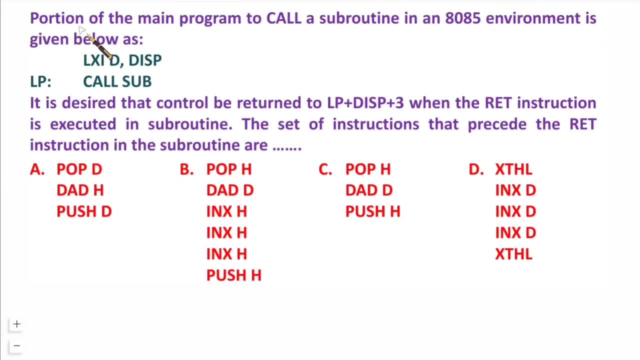 My dear students, now I will give you one very interesting question that will open up your mind regarding subroutine instructions. So question is: portion of the main program to call a subroutine in 8085 environment is given below. So here we have main program. 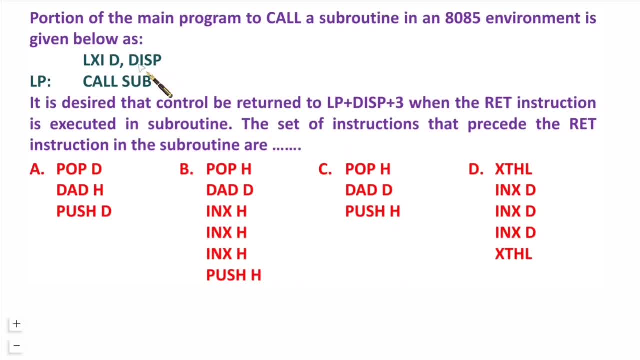 And you see what is written: LXID comma, DASP. So DASP, that is a label, right? This sub, that is also label, And this LP, that is also label. My dear students, you should know what is label. Label is address. 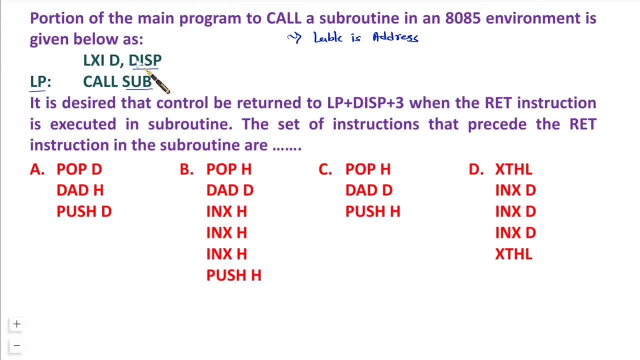 So here address is not given, It is given by label. So label will be 16 bits of address. that you should know. Now, when you write LXID, LXID, DASP, what will happen? Your DE register pair. that will get loaded as per this label. that is address. 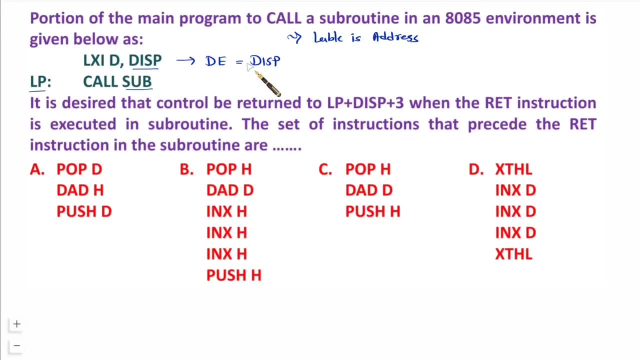 So I am writing DASP here. That will be address, but it is label right now. Now here what we do Call subroutine. Now you see this call, that is having actual address of LP And here sub is written. Means subroutine will get performed. 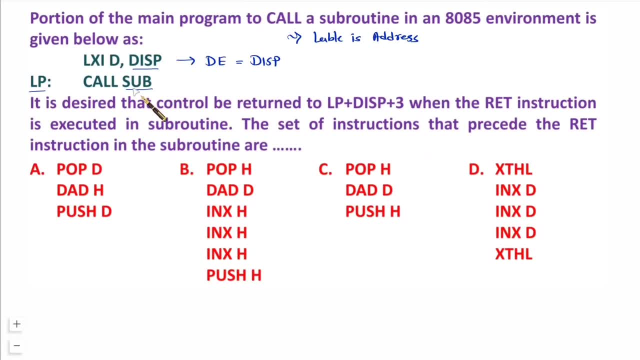 So when you execute call, what is happening? You should understand that. See, when you execute call, at that time next instruction address will get push on stack, So your stack will get modified, So stack, that will be next address instruction. 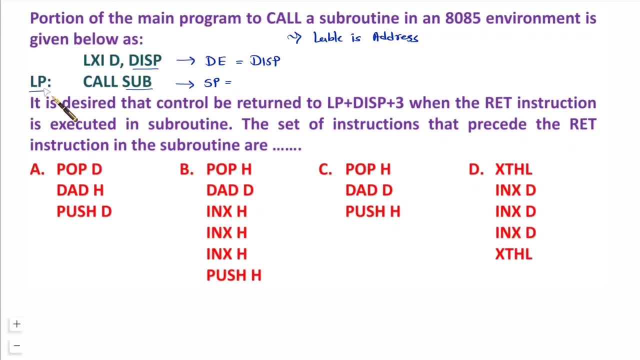 You see, call instruction address is LP, So call is 3 byte instruction. So next instruction should be having address, which will be LP, So stack pointer that will be getting loaded by LP plus 3.. Means program counters, main programs: instruction that we loaded on stack first. 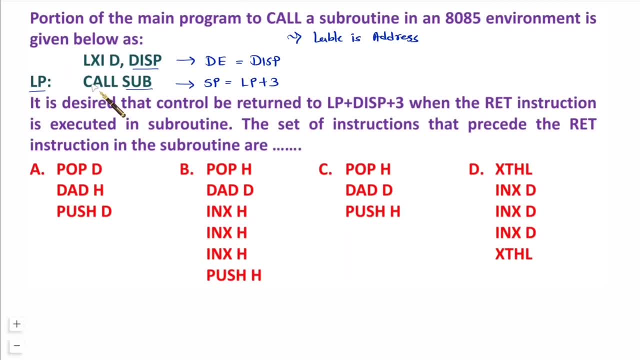 Right, When you perform call. After that we jump to subroutine. So stack pointer will be LP plus 3.. And now subroutine will get performed. Now it is desired that control to be written to LP plus DASP plus 3.. This is very essential, my dear students. 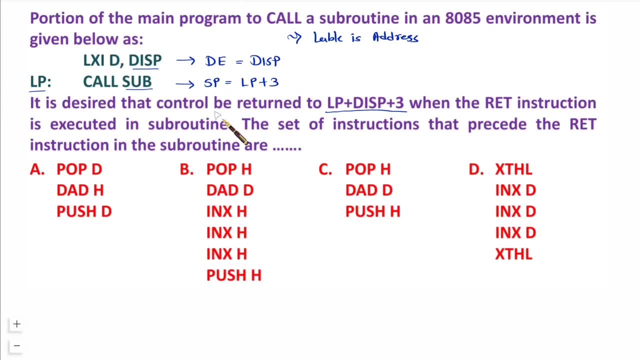 Programmer is telling you that it is desired to be written at LP plus DASP plus 3.. See normal subroutine will return at LP plus 3 over here, Which is next instruction after this call instruction. But it is desired to be written at this address. 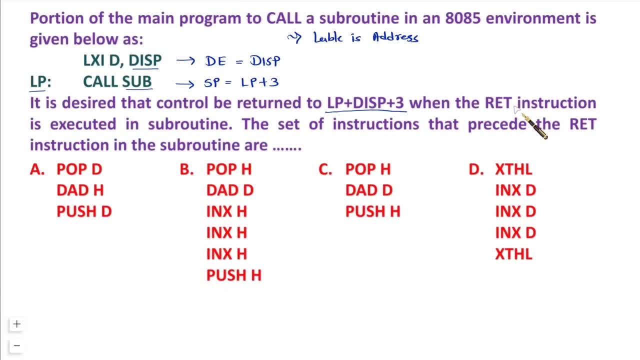 Which is LP plus DASP plus 3.. When return instruction is executed in subroutine, So the set of instruction that precede the return instruction in the subroutine are So which subroutine will follow this return execution? That is the question. So let us check it for all four programs, step by step. 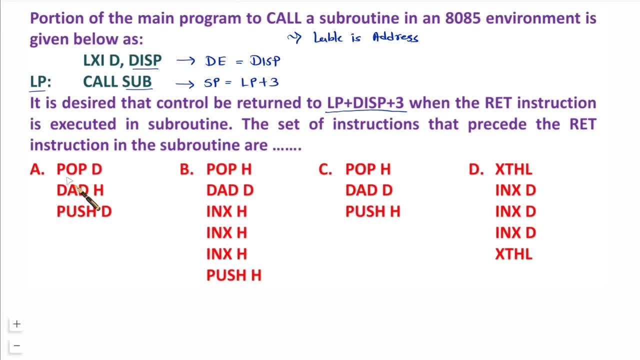 So first of all let us check it for option A. So here what we do is pop D. So after pop D, what will happen? Your DE resistor pair, that will be loaded by stack pointers data. That is LP plus. So here LP plus 3 that will go in DE. 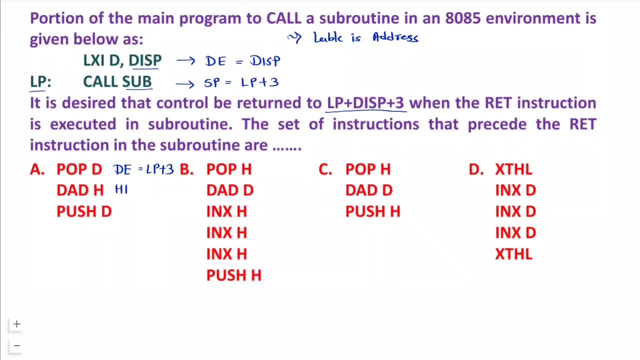 After that we perform dead edge. So dead edge means what HL resistor will be: HL plus HL, Right, So it will get 2 HL in HL after dead edge, And after that we perform push D, So this DE which is having LP plus 3.. 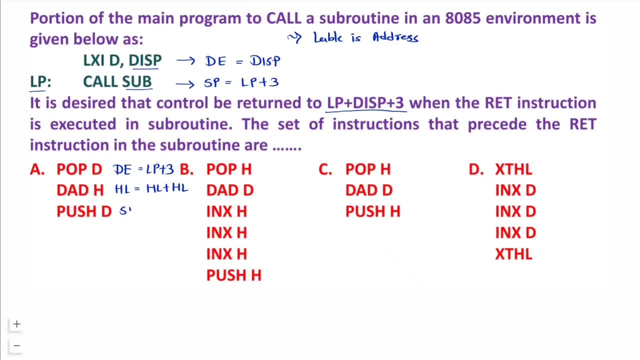 Now that we again push it on stack. So now stack will be having which data: LP plus 3. And after that, if you perform RET, Then return will execute which address, The address which is loaded by stack pointer. So return will execute this address. 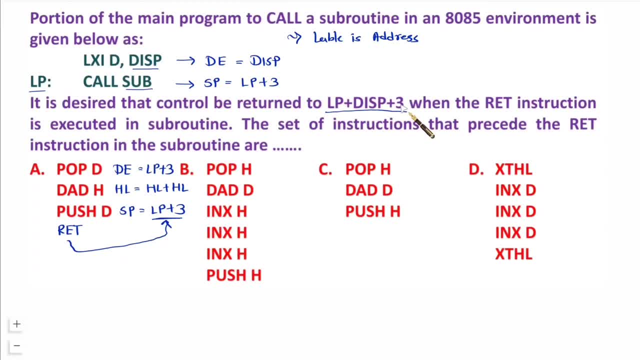 Now question is what We should execute: LP plus DISP plus 3 after return. So this is executing LP plus 3.. So this is false option. Let us see the option B. So when you perform POP H, What will happen? HL pair. 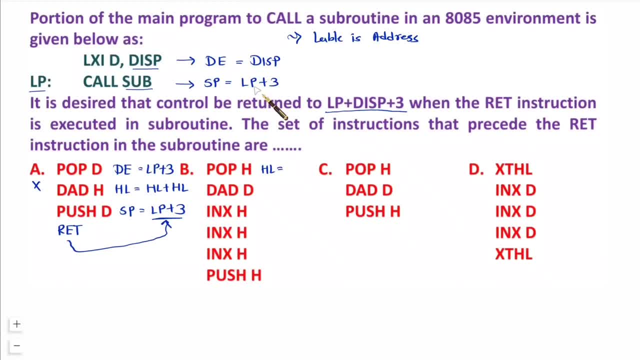 Now that will be taking data from stack. You see, stack is having LP plus 3.. So HL will be LP plus 3.. After that, we perform dead D. Now, when you perform dead D, What will happen? HL will be HL plus DE. 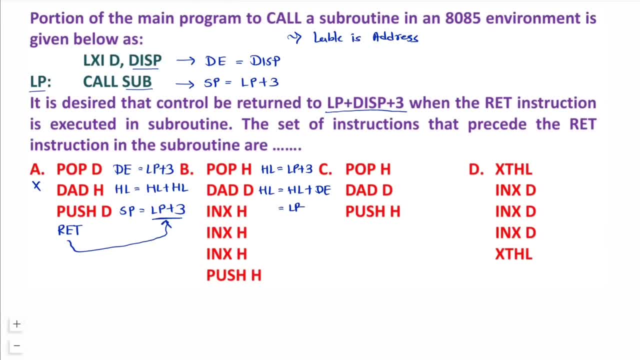 Now HL is how much LP plus 3. And what is DE? So you see, in main program DE is So LP plus 3 plus DISP. After that we increment HL 3 times. So as you increment HL 3 times, 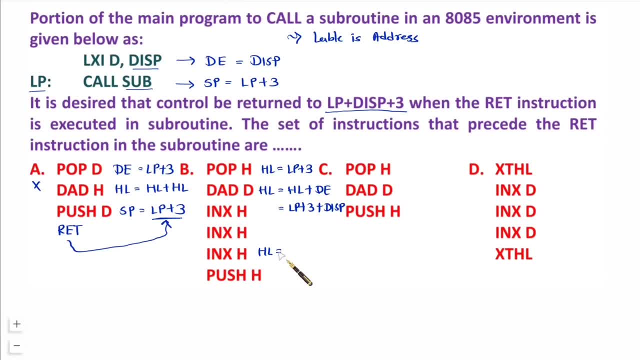 Here your HL will get modified to how much LP plus DISP plus 3 plus 3.. That will be 6.. And then you push H. So what will happen now? Stack pointer that will be having this data, That is, LP plus DISP plus 6.. 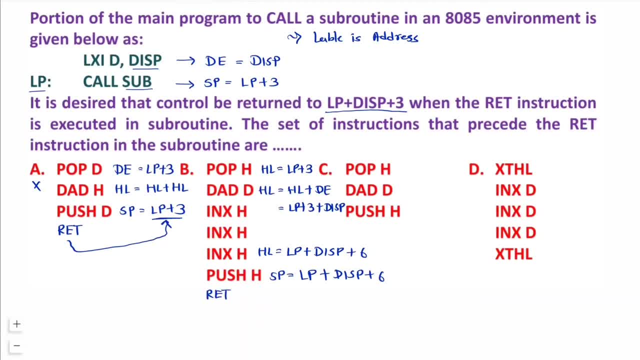 So once you perform return after this subroutine, This return that will happen at this address Which is there at stack pointer. So our question is LP plus DISP plus 3. Here SP is LP plus DISP plus 6. So this option is also false. 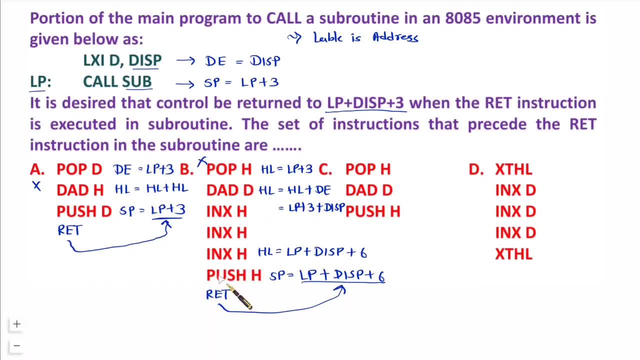 Now here. if you observe So same instructions are there Right? Only increment H that we don't do over here. So with this what will happen? HL will be LP plus 3.. Then dead H will make it to LP plus DISP plus 3.. 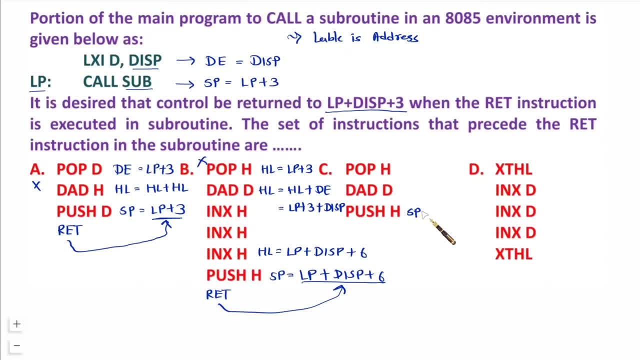 Then push H, That will gives SP is equals to LP plus DISP plus 3.. Right, It will not increment H 3 times here. So now, once you execute, return over here, It will be going to return at LP plus DISP plus 3.. 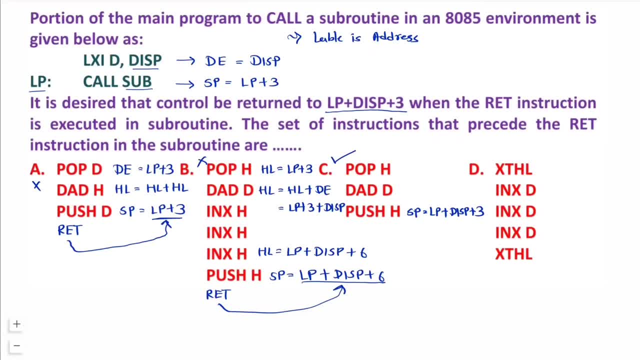 So this option is correct. Now, my dear students, Let us check it for option D also. So, with option D, XTHL is written. Now you should know what is XTHL. XTHL will exchange data of stack with HL. 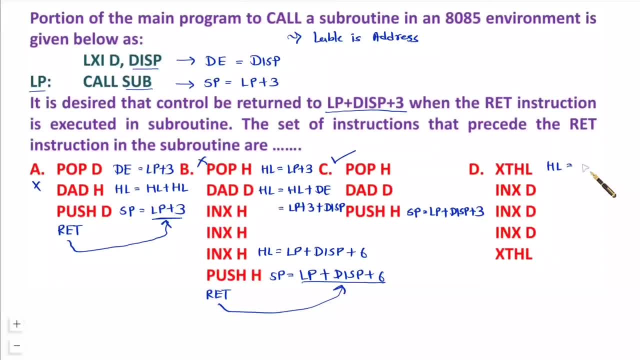 So now, what will happen? HL, Now that will be. You see, previously SP Was LP plus 3.. So HL will exchange SP And now HL will get to LP plus 3.. Right, So HL will be LP plus 3.. 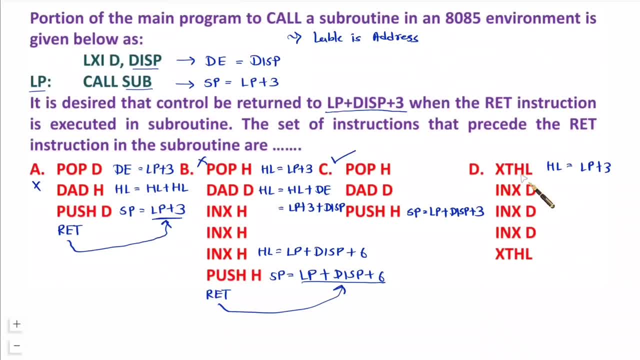 After exchange of data. XTHL means stack pointer. data will get exchange with HL pair. After that you increment D 3 times, So after that DE that will get changed. Initially it was DISP, So now after 3 increments It will be DISP plus 3.. 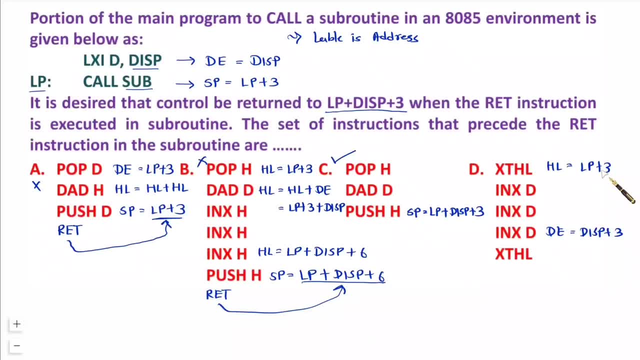 Again, if you perform XTHL, Then HL was LP plus 3.. So now stack pointer Now that will be LP plus 3.. Right, So once you perform return over here, It will get return at LP plus 3.. As stack pointer data is LP plus 3.. 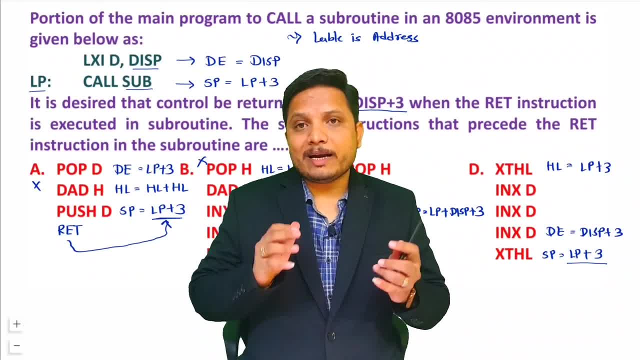 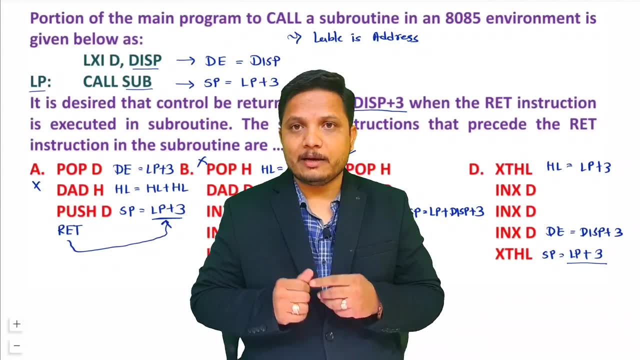 So this option is correct. So I think now, my dear students, You have a clear idea about How we should be using Call and subroutine, Right. So this type of trick equation may come in competitive examination. For that you should be ready.